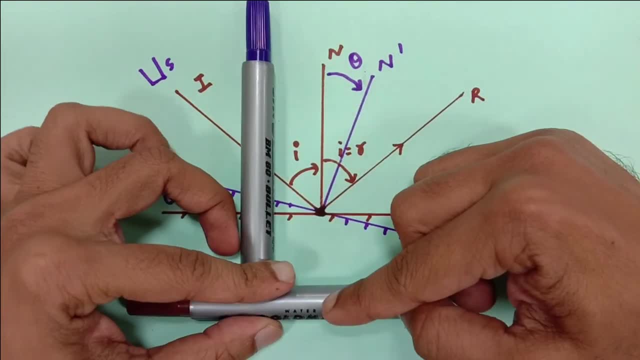 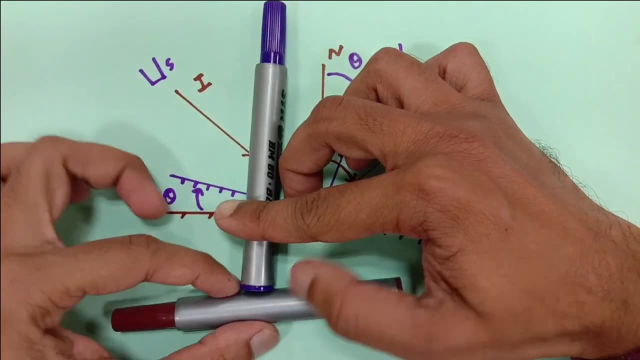 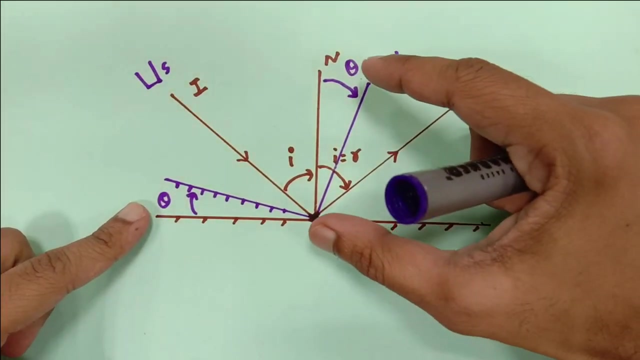 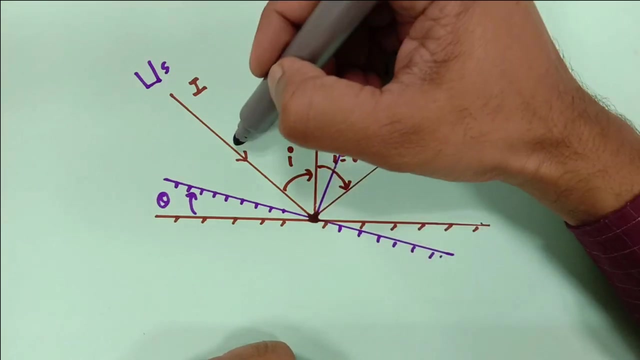 These are the two marker pens. This is my plane mirror. This is the normal. So if this turns by 30 degree in the upper direction, this will also turn by 30 degree in this direction. Like this, Correct? So the angle turns by theta. The normal also turns by the same angle. Now let's measure the new angle. 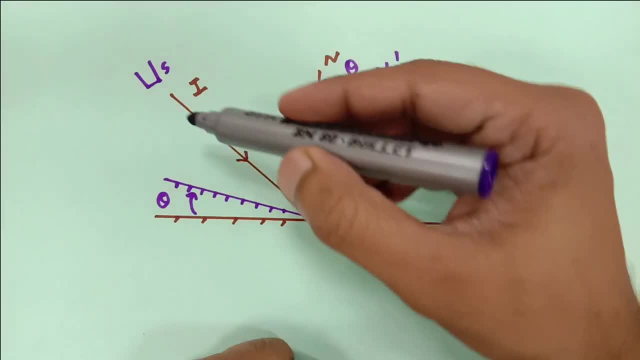 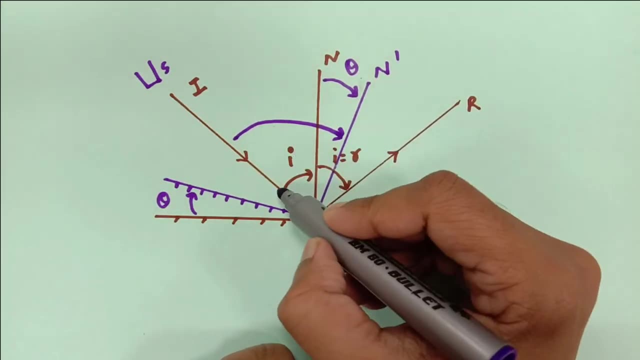 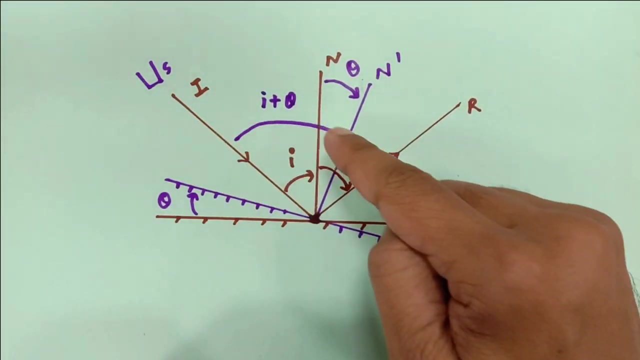 of incidence from the normal. The incident ray stays there itself. This is the new location of the normal and, as you can see that this angle is I, This angle is theta, So this angle is I plus theta. So now the new angle of incidence has increased by theta. So that means 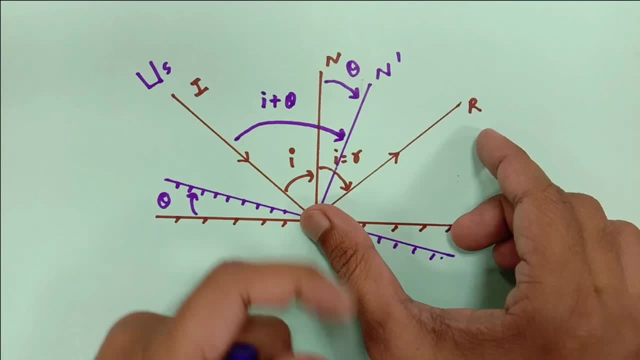 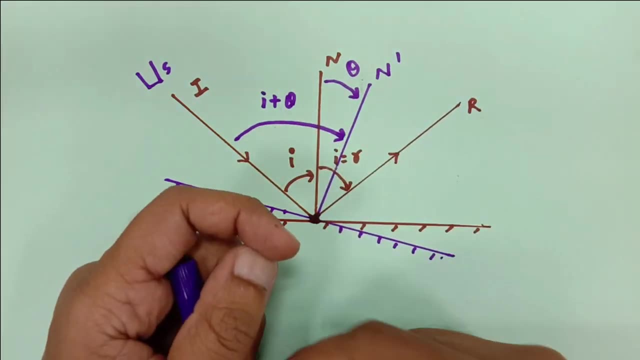 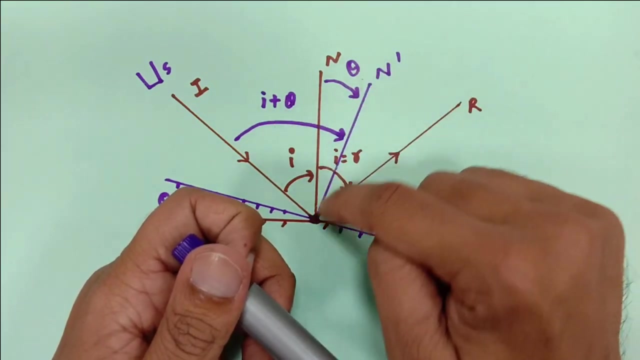 the new reflected ray should turn down, because earlier the angle of incidence was less, Angle of reflection was less. Now, if the angle of incidence has increased, so the angle of reflection must also increase, Because here the angle of reflection should be I plus theta from the normal. It is because the 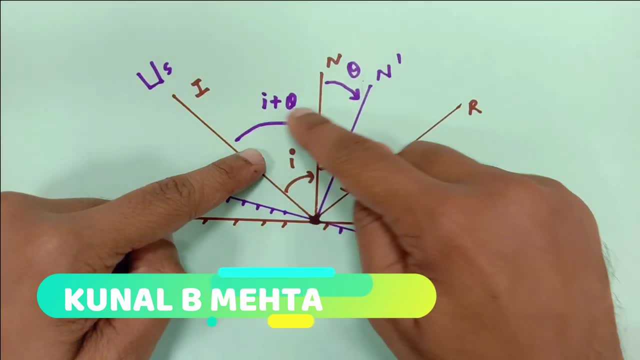 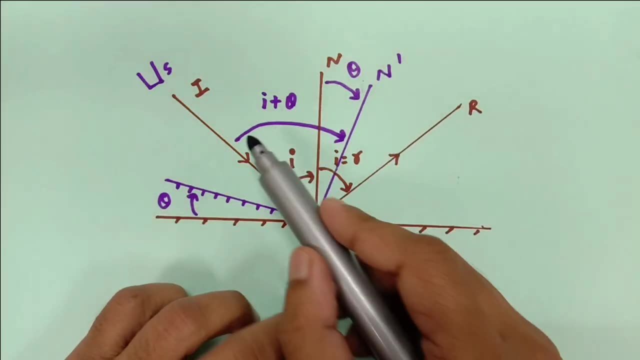 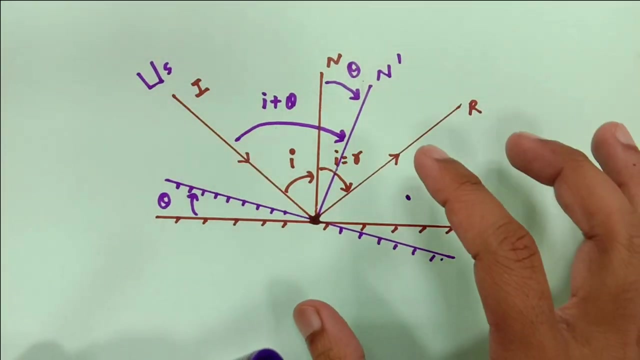 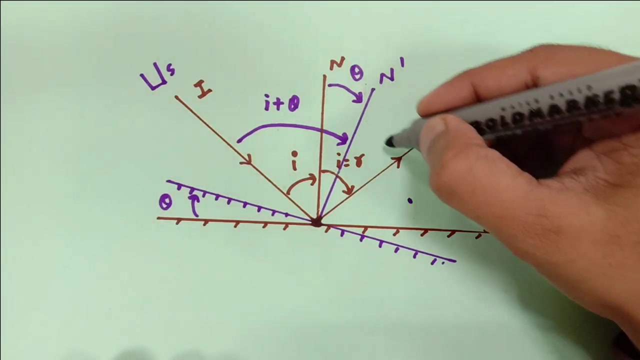 incident ray makes the same angle I plus theta which the reflected ray makes I plus same theta with the normal. So let me quickly judge that somewhere around over here the reflected ray should be. I'm just guessing. our diagram over here should not be very accurate in terms of angles, but if this angle is I plus theta, then this angle must be. 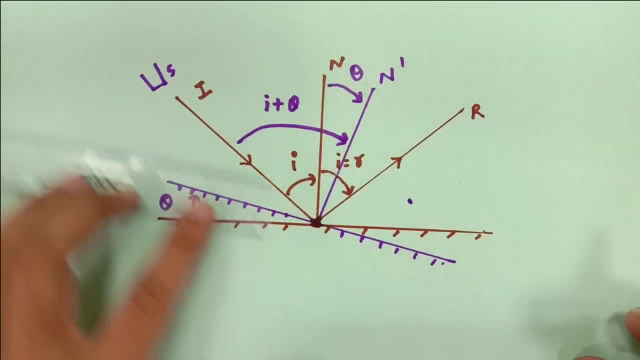 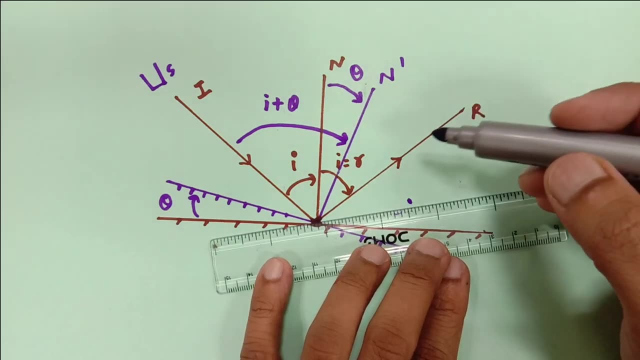 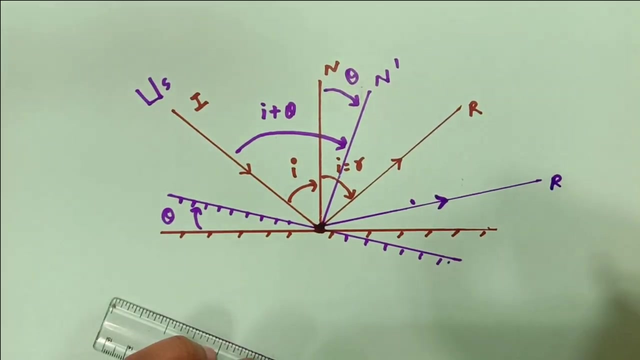 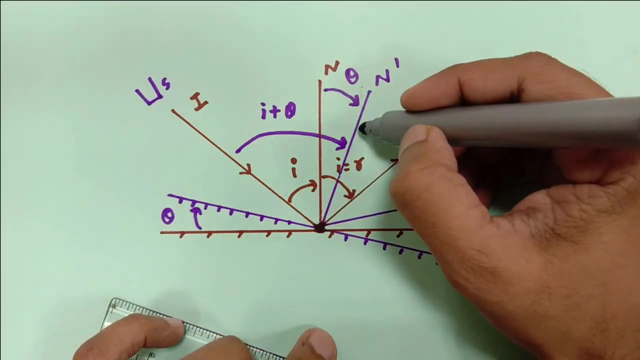 i plus theta from here. So let me draw this ray again like this: This is my new reflected ray over here. Let me call this as r dash. and I know that incident ray with respect to new normal it makes i plus theta, So the reflected ray must also make the same angle i plus theta, Correct? 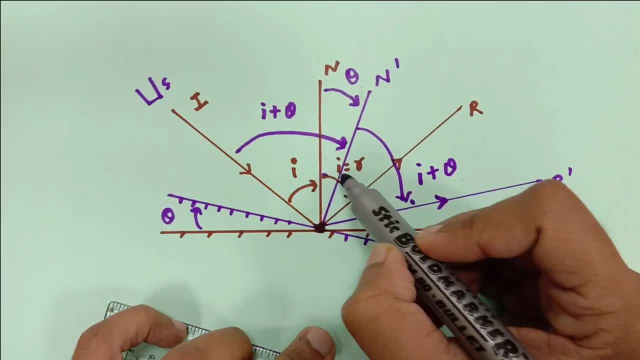 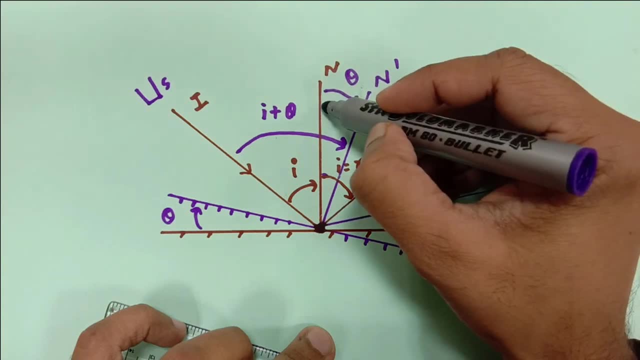 Now, people, we know that this angle is i. Actually it is r, but i and r are same. So if this is i, this whole angle, if this whole angle is i, because you look, this angle and this angle are same. This is theta.